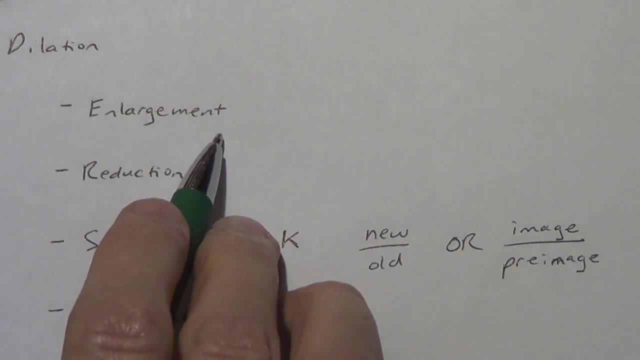 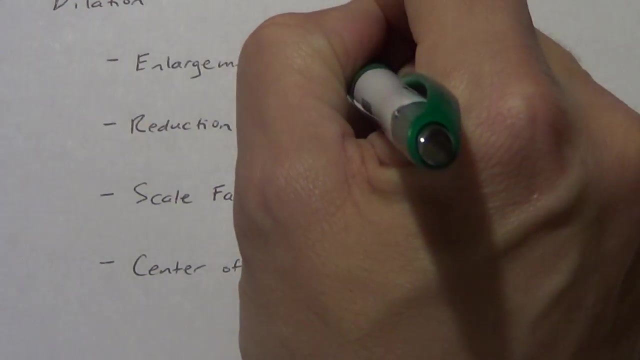 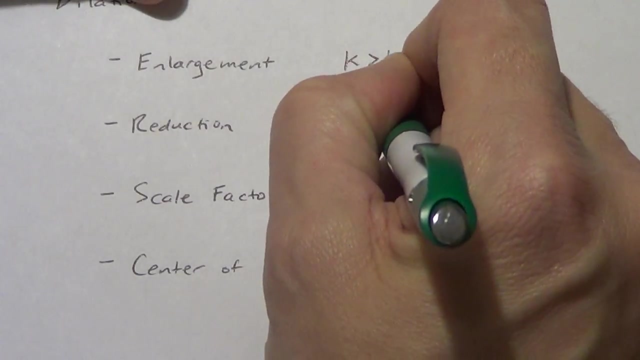 Okay, so a little review there. An enlargement meant that our shape got bigger. What about K? You guys remember what was true about K, K. with an enlargement, K was greater than 1, okay, Reduction, K was less than 1, but we also said it was greater than what number. 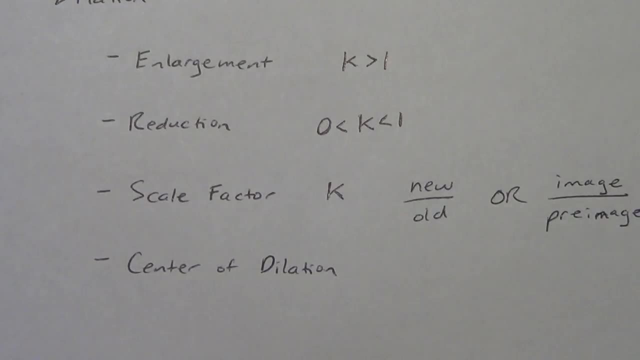 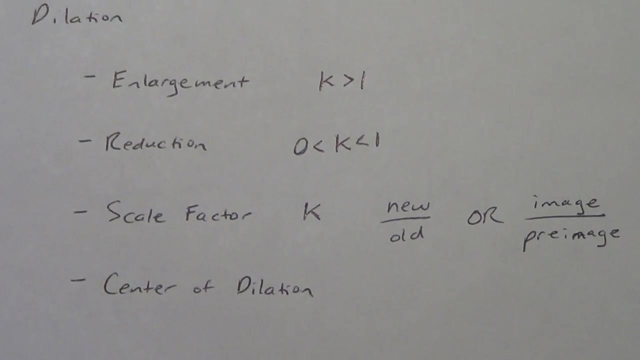 It was greater than 0. If you multiply everything by 0, you don't have anything left, so that doesn't make sense. And if you multiply by a negative, we get negative distances, which doesn't really make sense either. Okay, the center of dilation, remember, was where, if we connected the vertices, 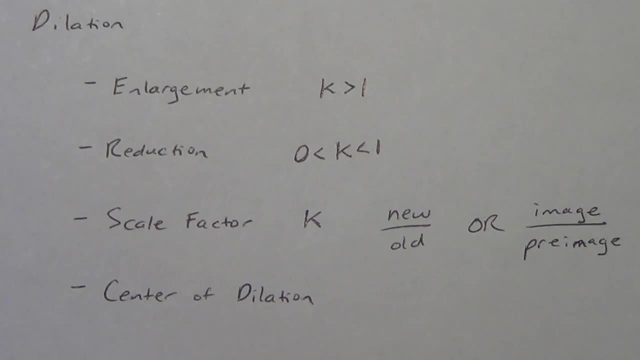 all of those little lines we drew would intersect at a single point, And that was the center of our dilation, Important concept for this lesson. unless I tell you otherwise, unless the book tells you otherwise, the center of dilation that you're going to use is going to be at 0, 0. 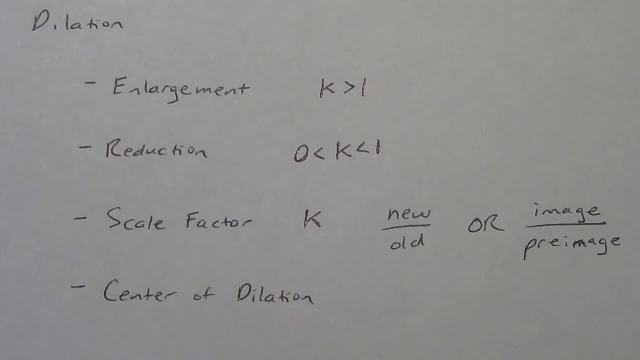 Okay, the fourth example I give you. it's going to be in the second video. I'm going to do an example where the center of dilation is not at 0, 0.. Okay, so that's the one. that's going to be a little bit different. 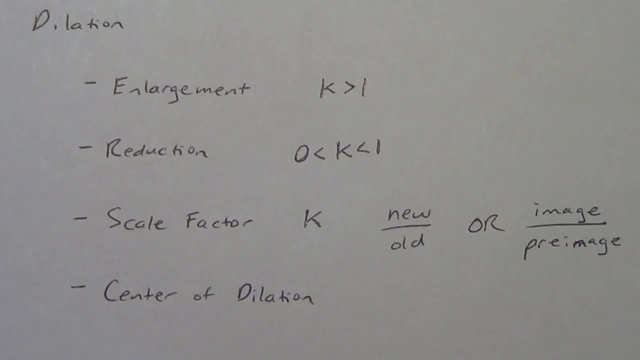 But most of the time, our center of dilation on a graph is going to be considered to be 0, 0, automatically, unless we tell you otherwise. All right, so let's take a look at the first example here. Okay, if you don't have graph paper, you need to get some graph paper. 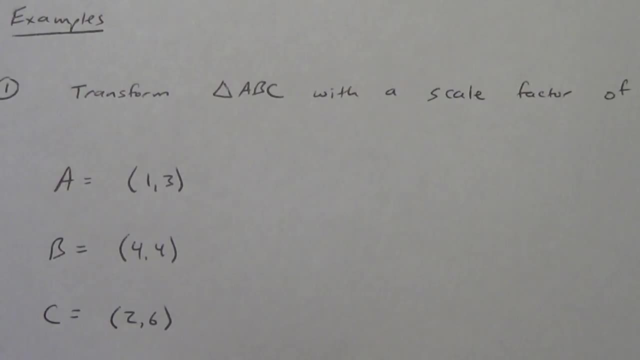 Okay, you can get it from me. If you really don't have any at home, go ahead. you can watch the video if you want kind of just follow along, but then I would recommend re-watching it when you have graph paper in front of you, so that you can actually graph things. 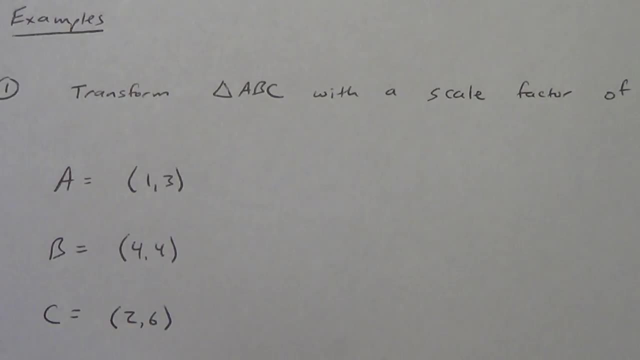 You can. if you don't have any at home, you have access to a printer at home. just go on The internet, type into some search engine printable graph paper, find a website that maybe has a PDF file or something like that that you can print. 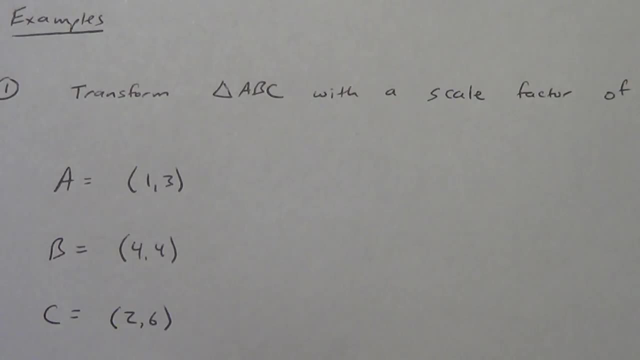 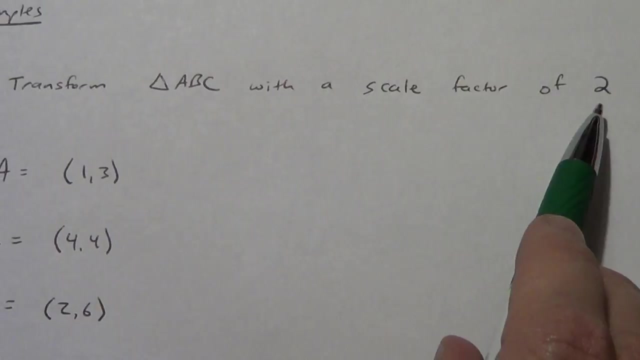 That's where I got mine, because I didn't bring any graph paper home with me tonight. All right, so all right, here we go. We're going to transform triangle ABC with a scale factor of 2.. Okay, a scale factor of 2, so K equals 2.. 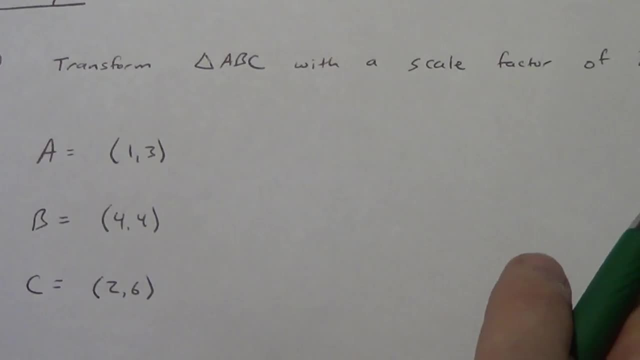 These are our three points. so go ahead and pause the video and graph those three points. Get them on your graph, Draw your triangle and while you're doing that, remember you can pause the video if you need to. all right, because I'm going to keep moving here pretty quick. 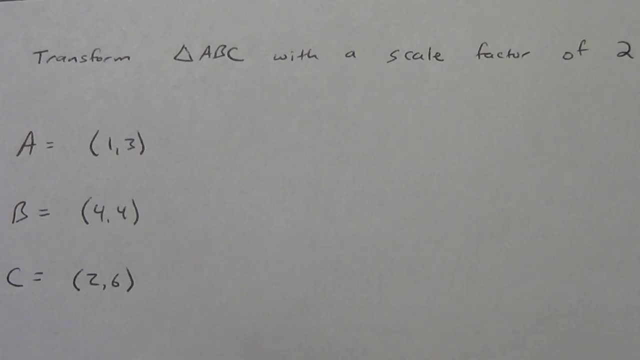 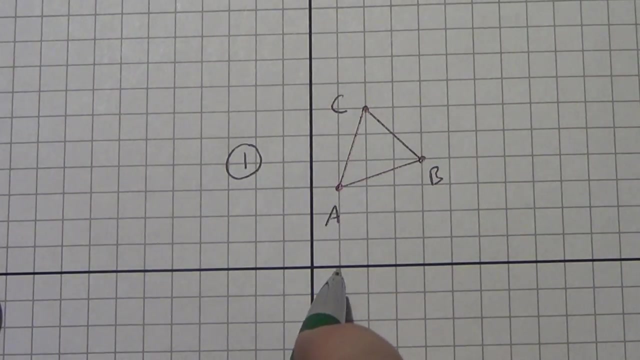 So 1, 3,, 4, 4, and 2, 6.. All right, if you graph those correctly, this is what your graph should look like. So I got this on my graph paper. All right, so we've got over 1, up 3, over to the right one because it was positive- up 3.. 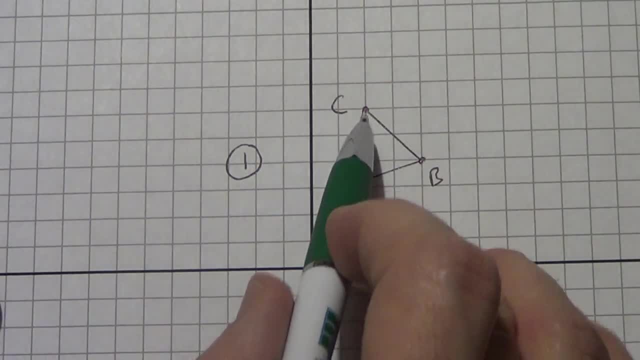 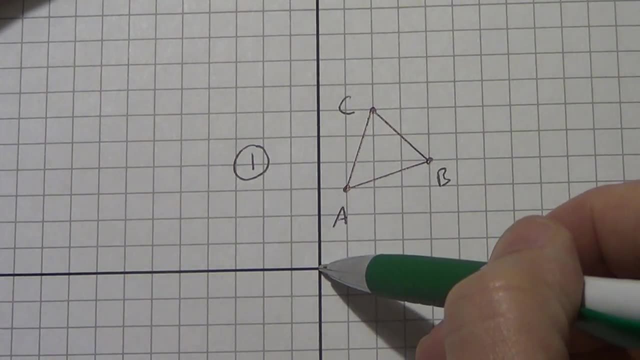 B- 4, 4.. B- 4, 4.. And C is over 2 and up 6, right 2 and up 6.. Okay, scale factor of 2.. What that means is that the distance from my center of my dilation to A. 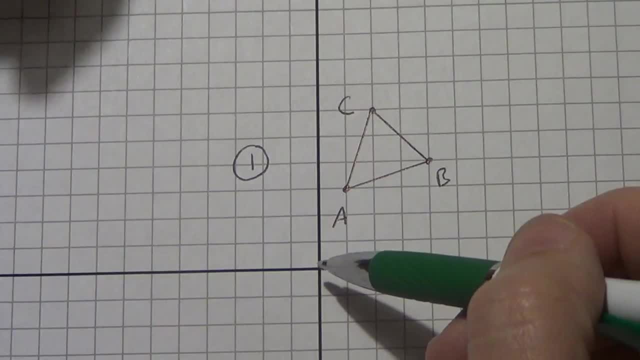 and then, when I do, to the next point, the one A is going to become, I have to go twice as long. So the easiest way to do that for right now is just to count. Okay, I'm going to show you a shortcut, though. in video 2. that works as long as the center of the dilation is at 0, 0. 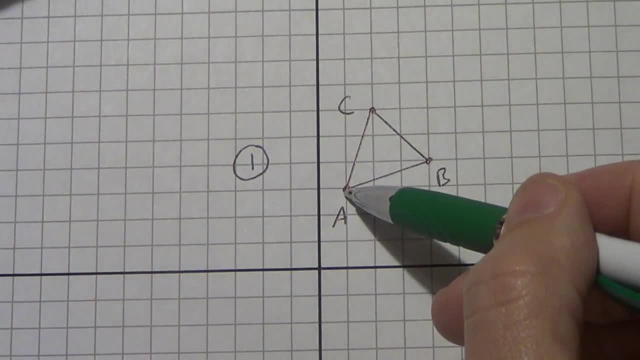 Okay, but for now we're going to count So right 1, up 2.. So scale factor is 2, so I have to double everything. So instead of right 1 and up 2,- or, sorry, up 3,, my bad- right 1 and up 3,, okay, I'm going to go right 2 and up 6.. 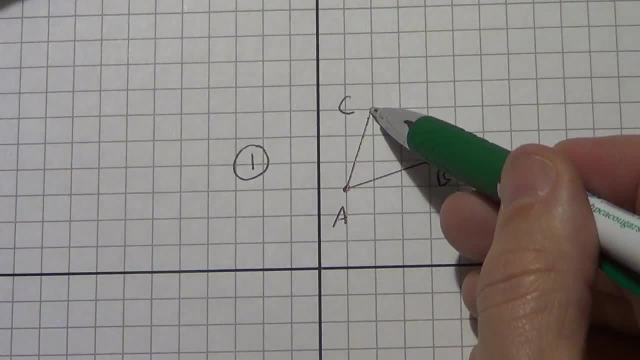 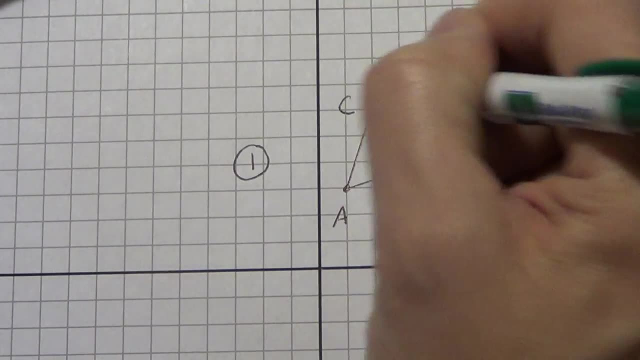 So right, 2 and up, 1, 2,, 3,, 4,, 5, 6.. Hey puts me at the same exact spot as C. Okay, that's fine. All that means is that this point, originally called C, is also going to be the new point where A is. 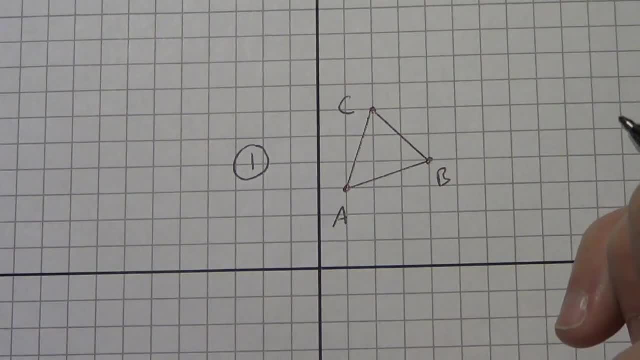 Now what do we want to call that In the book? sometimes they'll say something like this: Transform triangle AB. Transform triangle AB. C onto triangle DEF. Well, in that case, A was first, D was first. I would call it D. 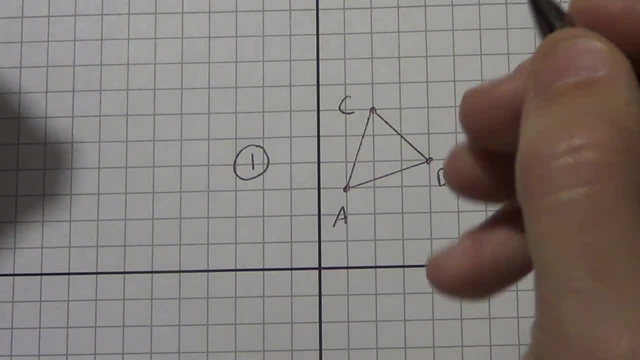 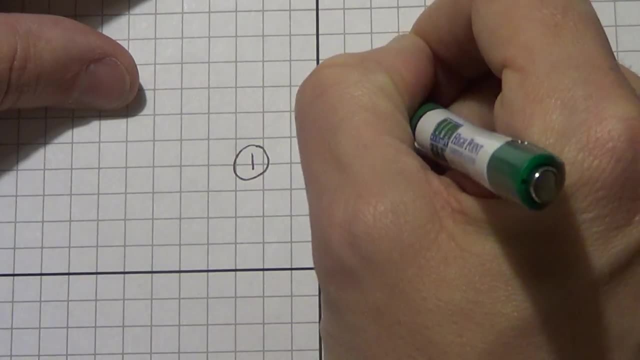 I didn't really tell you what to call the new triangle, So what I want you to do is use the prime marks. We did this before, So I want you to call this point right here A prime. okay, So that point right. there is both C. 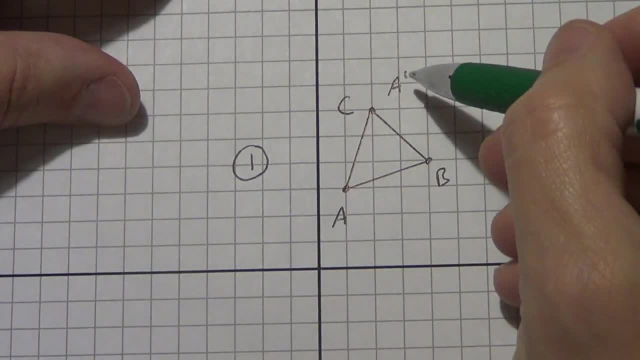 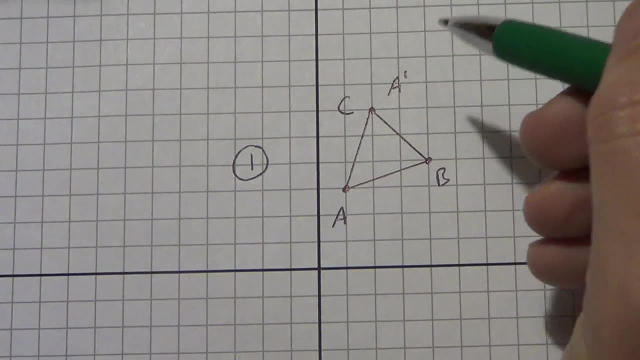 It's the original C and it's the new A. Remember, the prime mark means the A means it's related to A came from A, but prime means it's its own unique thing. I kind of talked about this like somebody who has the name of Junior. 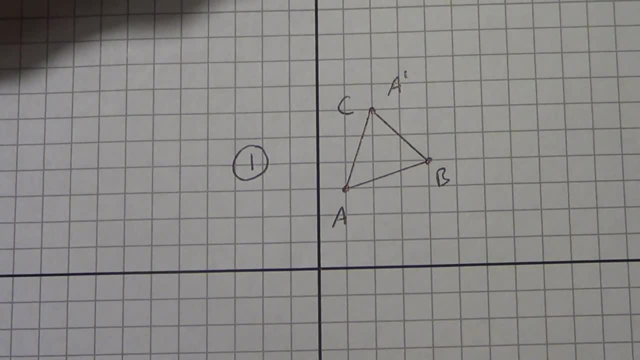 I talked about that in class. So if someone has the name of Junior, all right, we know they're related to somebody else, They came from someone else, all right, but they're their own unique person as well. okay. So A prime says, hey, it's related to A. 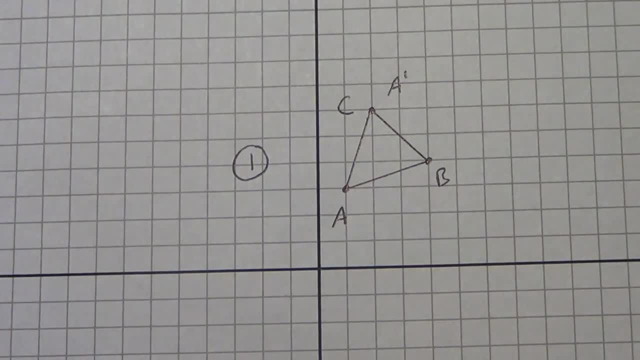 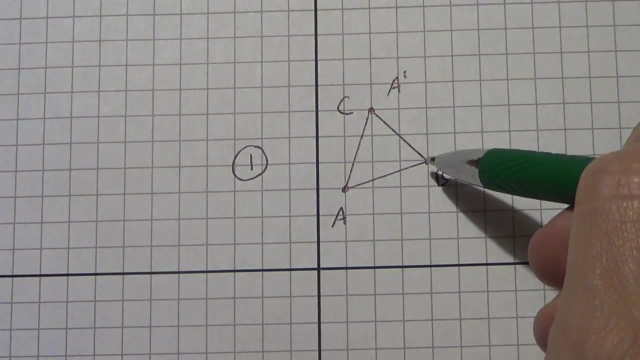 It came from A, but the prime mark tells me it's its own unique point, It's in a different place. all right, Okay, let's go to B. So to get to B, I go right, four and up four. Remember scale factor of two. so I double everything. 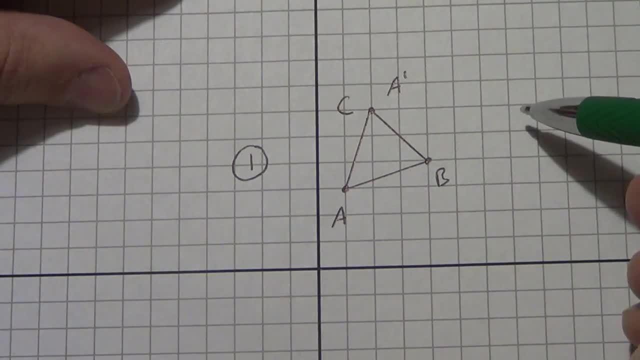 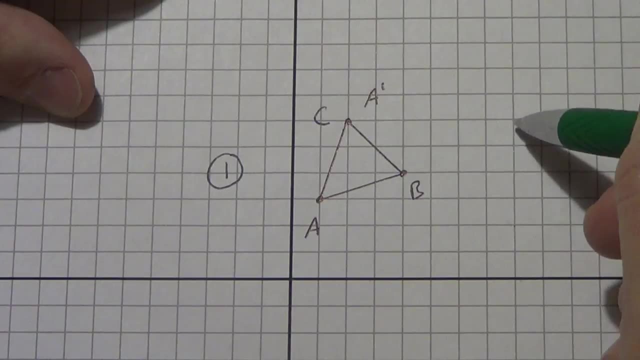 So I got to go eight and eight. So right, eight, Right eight and up eight. okay, So let's count that out: One, two, three, four, five, six, seven, eight. One two, three, four, five, six, seven, eight. 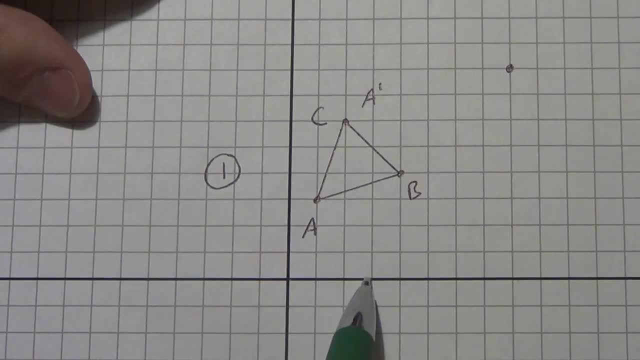 I'm going to put my dot there. I'm going to double check my counting: One, two, three, four, five, six, seven, eight. One, two, three, four, five, six, seven, eight. Okay, we're good. 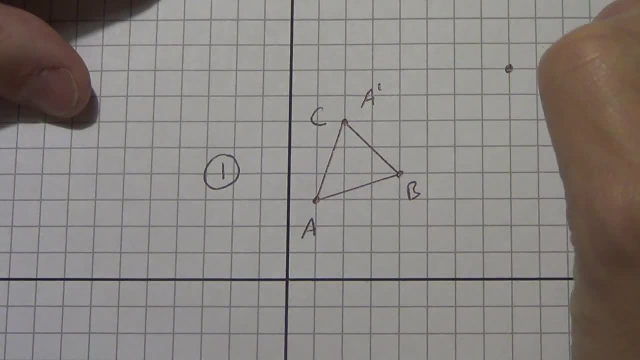 Now, if that was B, what are we going to call this point up here? Okay, we're going to call it B prime. Okay, let's talk C, Right, two and up six. So what do you think we should do? 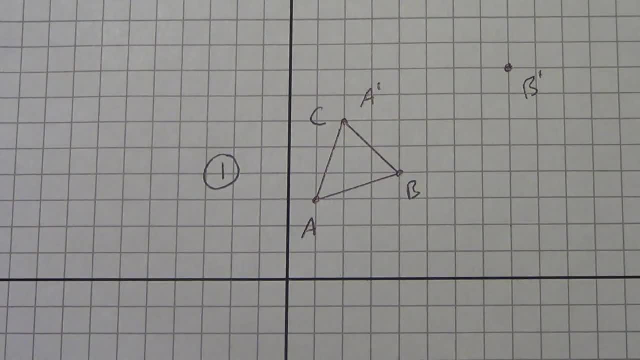 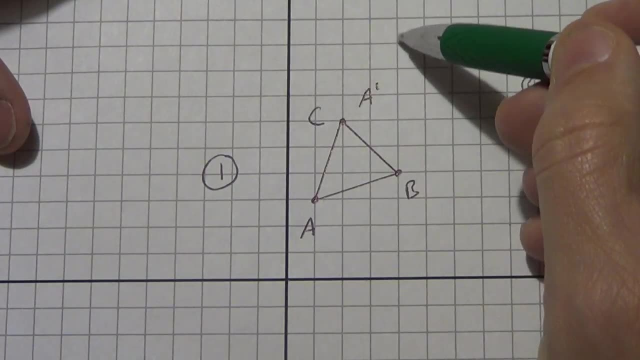 Scale factor of two Right, two, up six. We got to double everything, So right, four and up 12.. One, two, three, four. One two, three, four, five, six, seven, eight, nine, 10,, 11,, 12.. 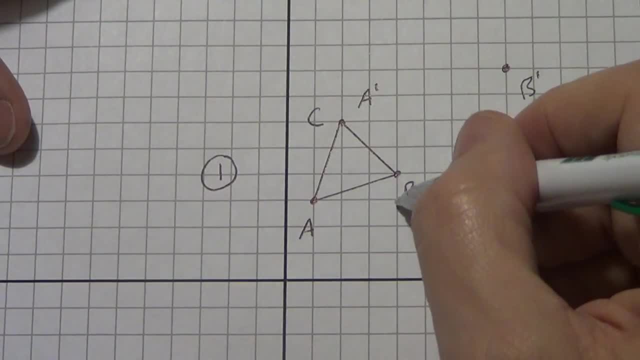 I'm going to double check that real quick: One, two, three, four. One two three, four, five, six, seven, eight, nine, 10,, 11, and 12.. Again, that was C. 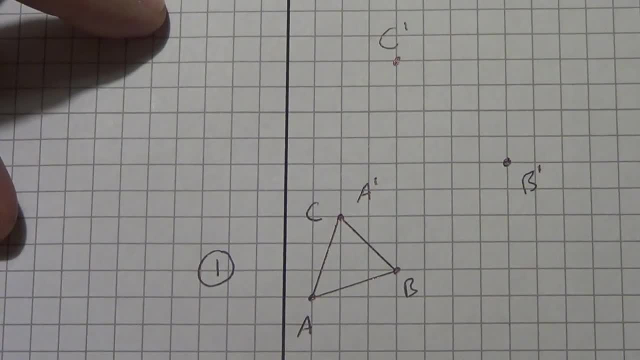 So I'm going to call this one up here, C prime. Sorry, it went off the camera there for a second. All right, so now I have my three points: A prime, B, prime, C, prime, graph. I'm going to draw my triangle. 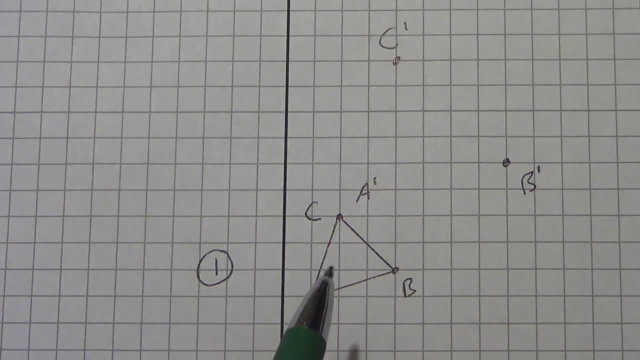 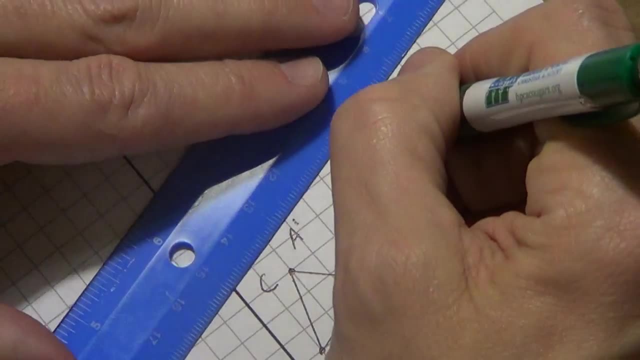 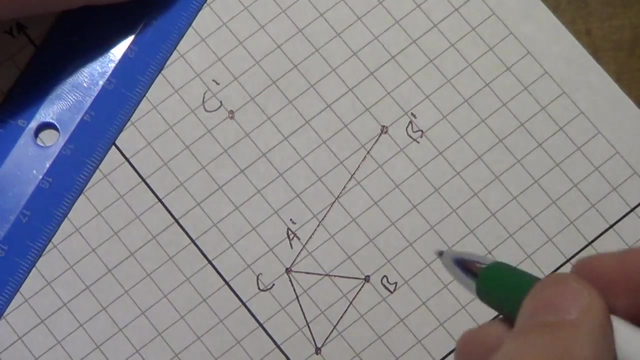 And, if I did this correctly, the new triangle should look what to the original triangle? It should look similar. Okay, if they don't look similar, I did something wrong. Okay, so here we go. A prime to B prime. Now, another thing that should be true is that when I draw this A prime, B prime segment, 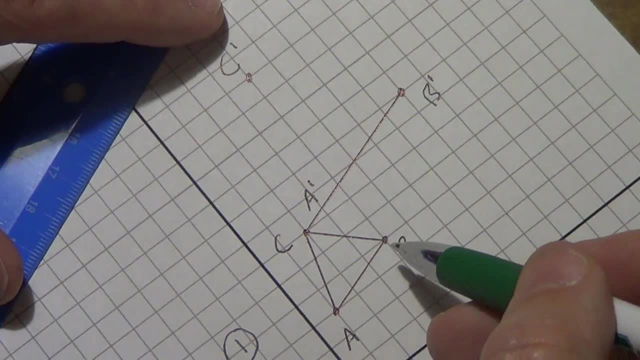 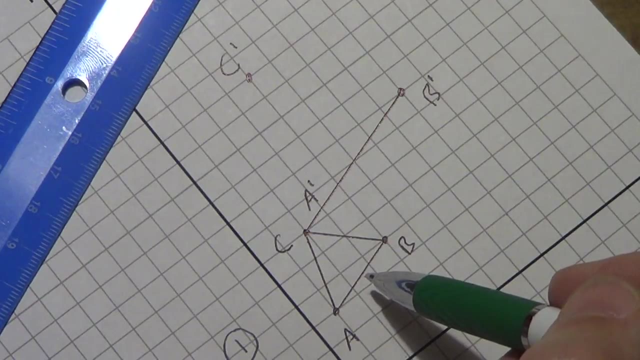 it should be parallel to the AB segment And it should be twice as long because my scale factor is two, They look pretty parallel. I could check parallel by doing slope, Remember rise over run. Or we can do Y2 minus Y1 over X2 minus X1.. 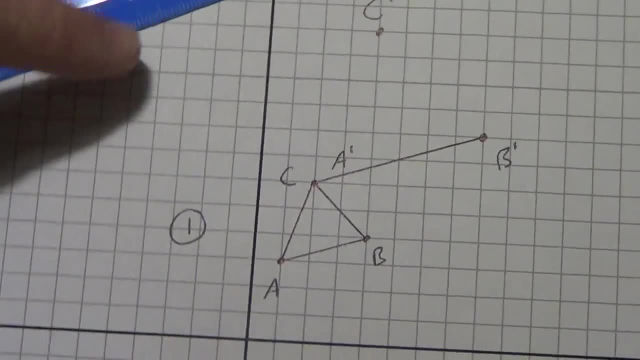 And as long as those slopes reduce to the same thing, I'm fine. So let's check that real quick. Slope rise over run, Rise of one run of three. It's going up, so it's positive. So that's a slope of one third. 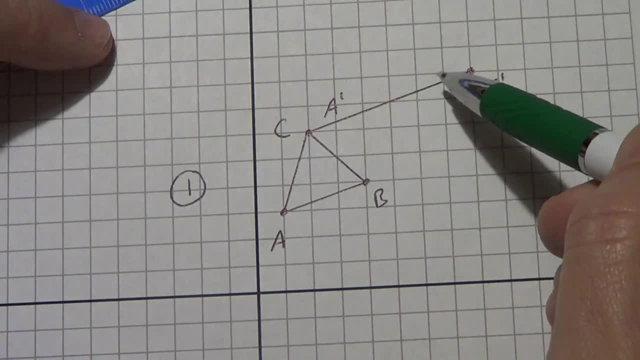 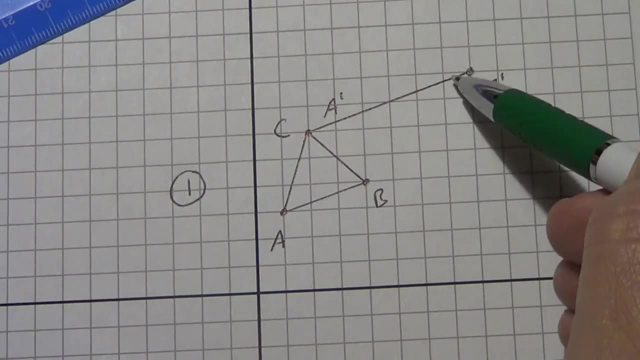 All right, here up two, One, two, three, four, five, six, right six. So that's a slope of two sixths which reduces to one third. So this slope is one third. This slope is one third. 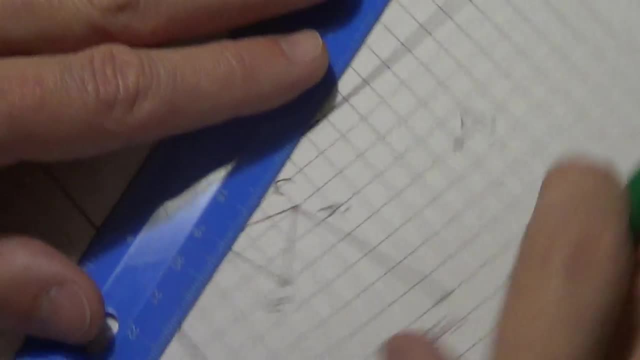 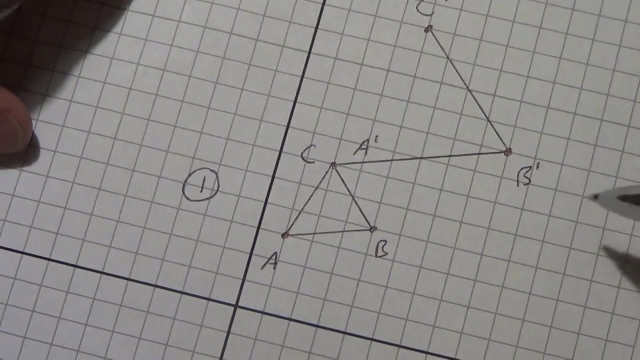 They're definitely parallel. Good tells me I'm doing something right. OK, let's connect B prime to C prime. I'm not going to bother checking the slope. I'm going to take a quick look and see if it looks pretty parallel. 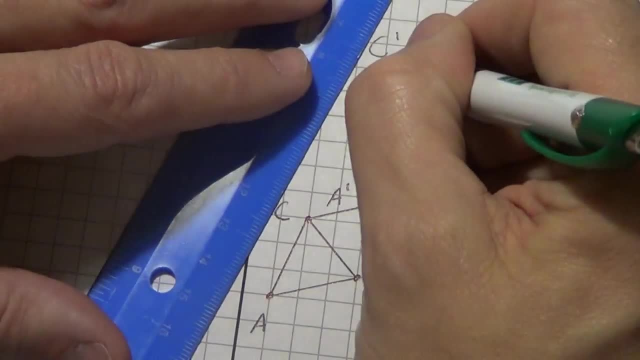 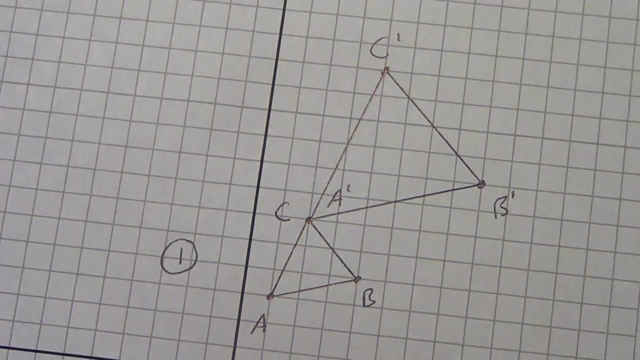 It does OK. so I'm not going to do the counting, though, on that one. just to save some time for right now, Let's connect C prime to C And we have our new triangle: A prime, B prime, C prime. 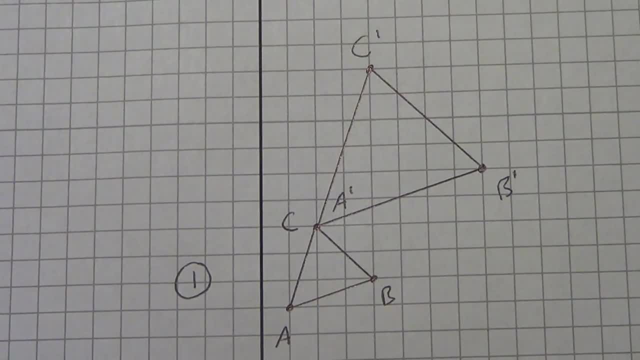 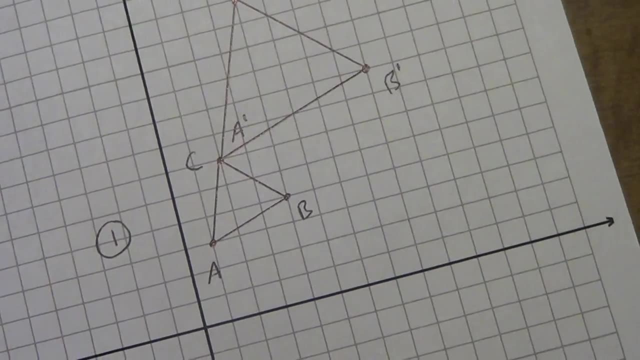 Does it look twice as big as the original? It should. OK, every distance is twice as long. Keep in mind that if we drew the dotted, I'm going to do this on another one, But if I drew the dotted lines to connect the vertices, 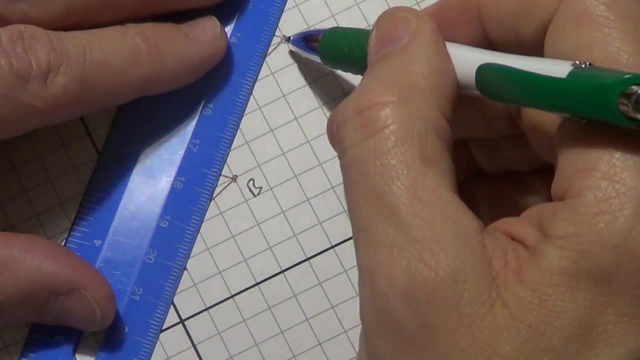 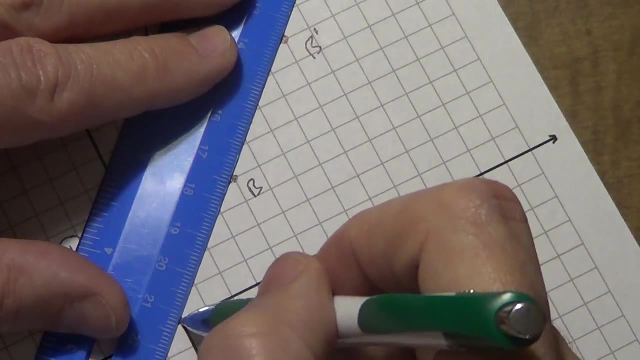 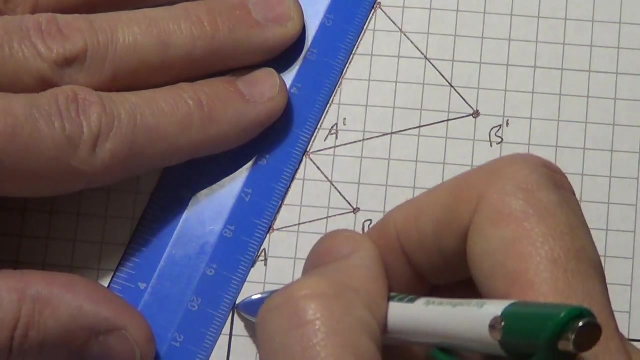 it should lead back to my center. I'm just going to show you how that would work on this by lining it up: B prime, B, and you'll notice it comes right through my origin. OK, let's go with A? prime and A, A, prime and A and right through my origin. 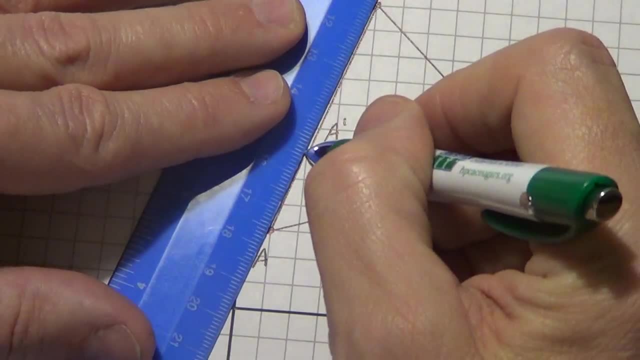 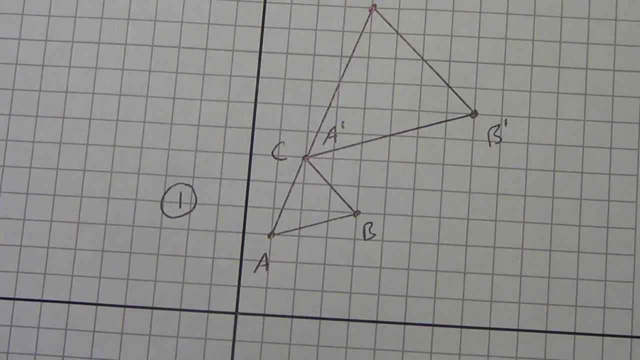 if I were to actually connect it. Same thing up here, C prime with C, and right through my origin, if I was to connect it. OK, So this is making sense, 0,, 0 being the center of my dilation. OK, The other thing I want you to be able to do is write those points down. 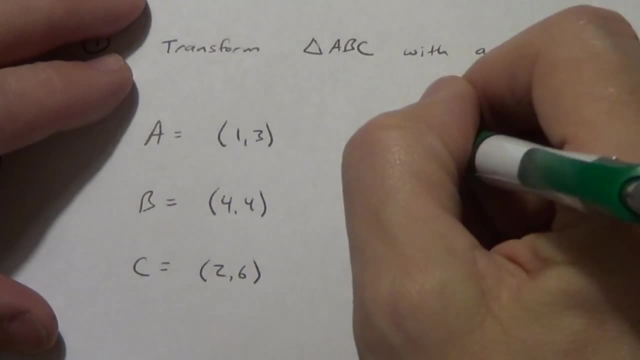 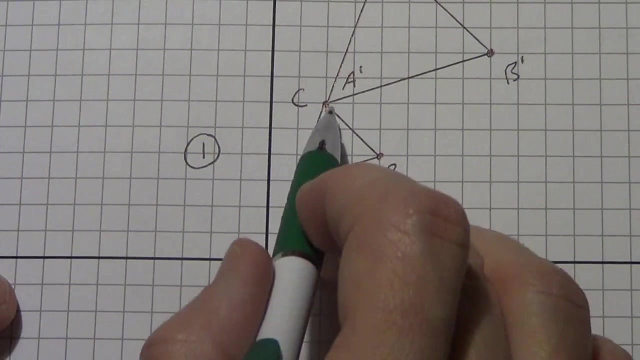 So let's go back to this other sheet: A prime, B prime and C prime. So A prime. remember, if we look back, where that was, it was over 2 to the right and up 6. That's the point 2, 6.. 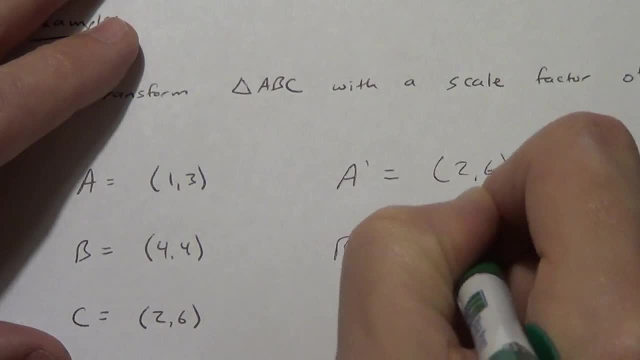 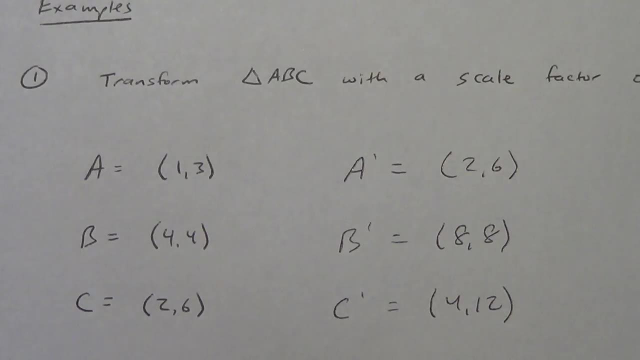 B was right: 8 and up 8, so that's 8, 8.. And C, prime, was right: 4 and up 12.. OK, There we go. OK, So that's the end of video 1.. Make sure you watch video 2 as well. 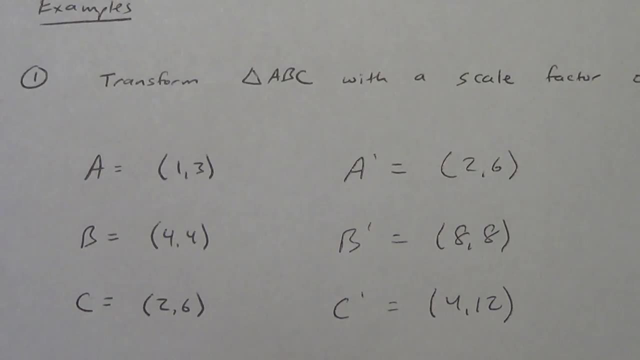 I'm going to teach you a quick shortcut right at the beginning of the video And then remember the fourth example. So I'm going to do a second, a third and a fourth. The fourth example: we're going to have a center other than 0, 0.. 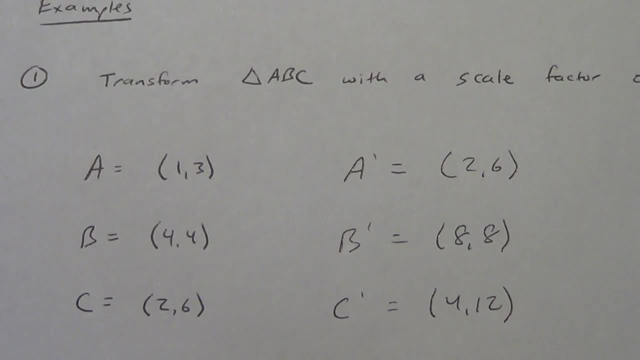 It does make it a little harder because we won't be able to use the shortcut, So make sure you watch both videos.